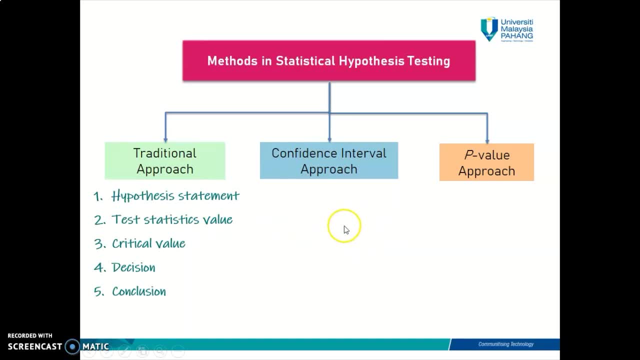 confidence interval approach, you will have similar steps but a little bit different. In confidence interval approach, there are only four steps that you need to do. So in confidence interval approach, there are only four steps that you need to do. The first one is very much similar to the one in the traditional approach, which is you need to. 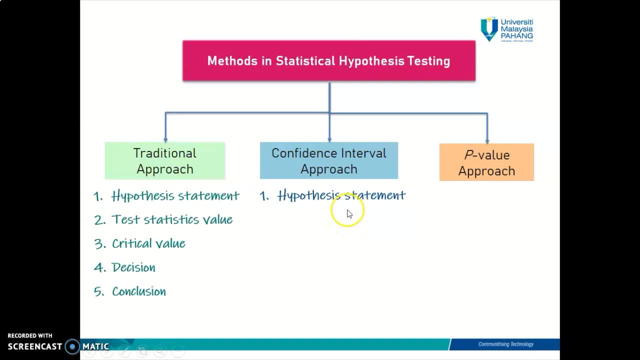 construct your hypothesis statement from your claim. You need to come up with HNL and also H1. And it's exactly the same step as in the traditional approach. okay, So the second step is to find the confidence interval which is appropriate or which is relevant to your. 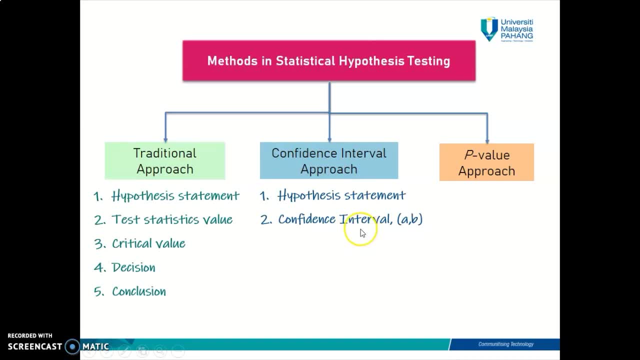 claim. So this confidence interval in step two here is the exact same confidence interval that you learned in chapter two. So this is where you get to apply what you learned in chapter two in hypothesis testing. okay, And the third step here is different from the traditional approach. 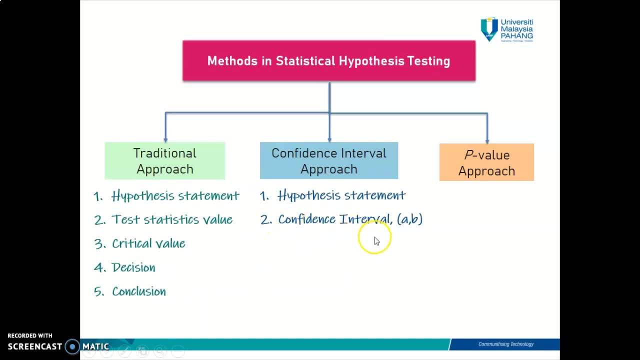 You no longer need to establish any critical value. The third step in confidence interval approach: you can straight away make your decision. It's the same decision that you had to do in the traditional approach. It is whether to reject HNL or to do not reject HNL. But the rules here will be a bit different from the traditional approach. 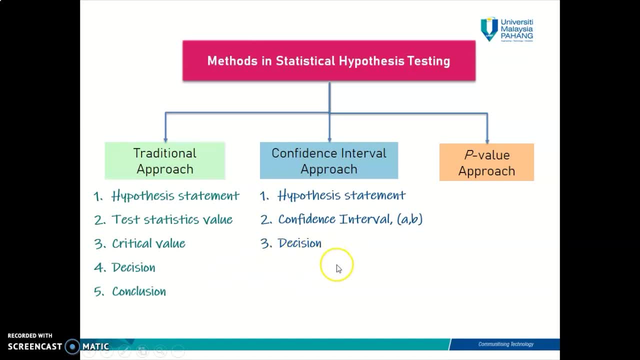 and we will go to that later. right And finally, after making your decision, you need to make a conclusion about your claim: whether you have enough evidence to support your claim, or is it? you have enough evidence to reject your claim and whatnot? okay, So the second step is to make your decision. 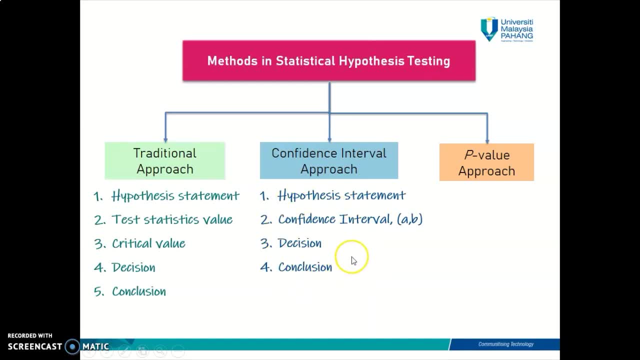 So these are the four steps in hypothesis testing using confidence interval approach. I have one good news for you, because in confidence interval approach it is only applicable for a two-tail test- hypothesis testing. So you no longer need to worry about whether it is this a one-tail. 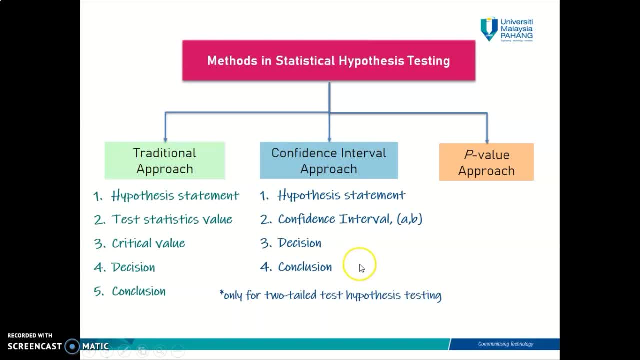 test. Is it a two-tail test? You can only conduct a hypothesis testing using confidence interval approach claim if your hypothesis involves a two-tail test. all right, okay, so that's pretty clear. all right, so let's discuss about step. okay, so let's talk about how to make decision using. 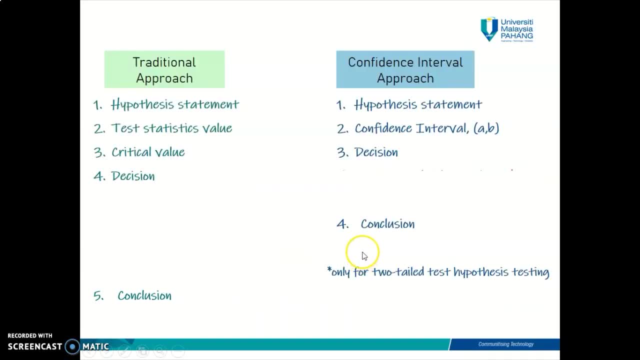 confidence interval approach right. so i'm going to make a comparison between the traditional approach- decision making- and the confidence interval approach- division making- so that you can have a better understanding about the differences between the two methods. okay, so previously, in the traditional approach, how do you make decision whether or not to reject or to do not reflect? 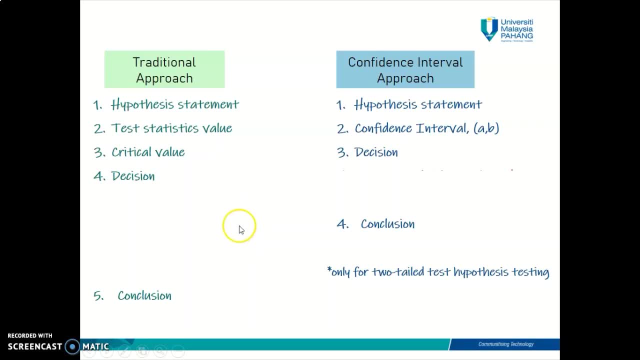 now? well, it's based on your test statistic values, right, you will. if your test statistic value falls in the rejection region, you will reject h now. so that is in traditional approach. but what about in the confidence interval approach? well, in confidence interval approach, it depends on your hypothesized parameter. yes, it depends on your hypothesized parameter. 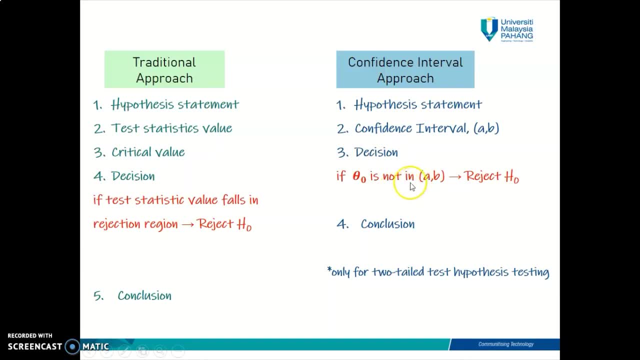 if your hypothesized parameter is not included, it is not in the confidence interval which you obtain in step two, so your decision will be to reject h now. okay, so this is a little bit different from the traditional approach. in the traditional approach you will be looking at the test statistic value, but in the confidence 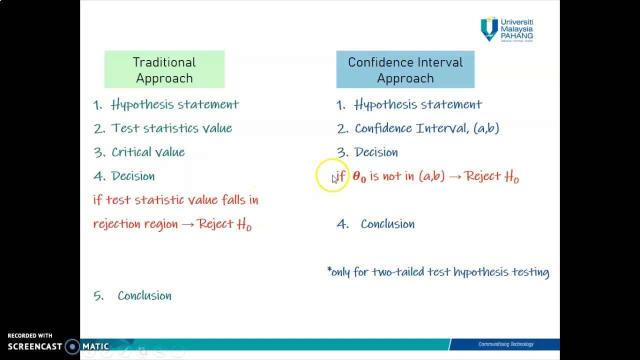 interval approach, you'll be looking at the hypothesized parameter value, right? so that is how to decide to reject h now. so conversely, if you wanna, if your test statistic value falls in the acceptance region, you would need to do not reject h now in the traditional approach, while in the 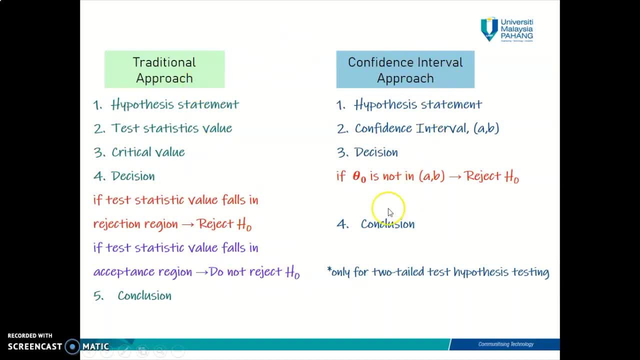 traditional approach, you will be looking at the hypothesis value, while in the confidence interval approach, if your hypothesized parameter is in the confidence interval obtained in step two, then your decision is to do not reject h now. okay, so i think that is pretty clear. um, you need to remember these rules for confidence interval approach and 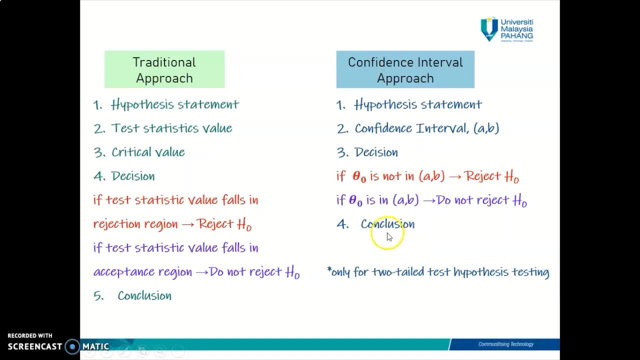 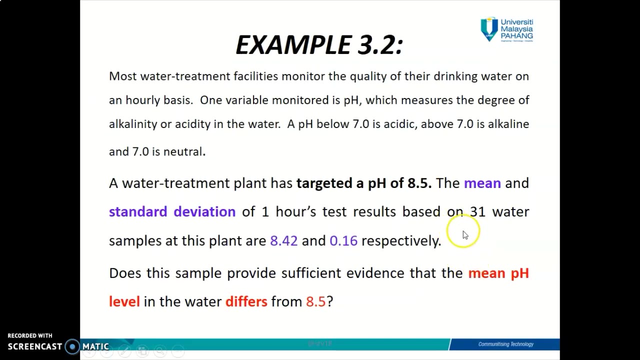 conclusion is the exact same conclusion which you also did for traditional approach. okay, so why don't we jump to our first example for this video, i'm gonna recycle the same example we use in chapter 3.2, so this is the exact same example, but we're gonna solve this using the 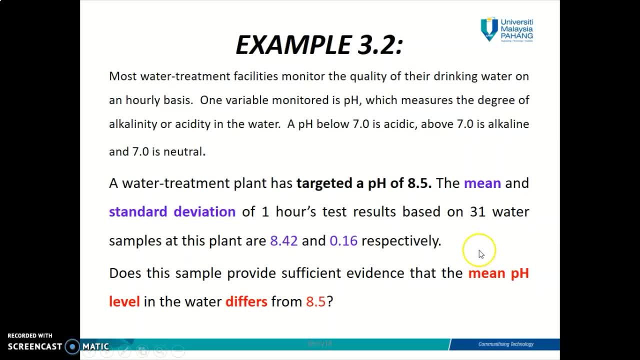 confidence interval approach. previously, in chapter 3.2, we solved this using the traditional approach with all the five steps, but now in this video, we're gonna solve this same question using the confidence interval approach, and then we're gonna solve this using the confidence interval approach. 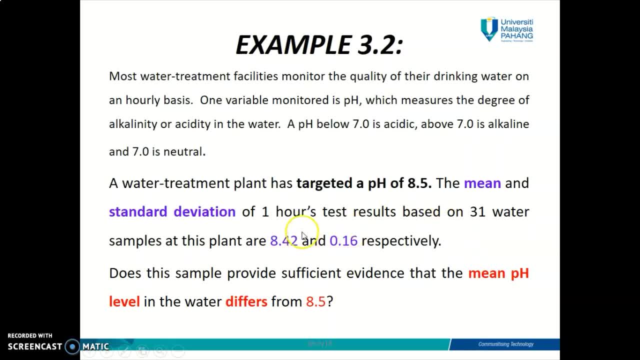 Okay, so these are the information obtained from the question. They provide you with the mean and standard deviation of the sample. Okay, 31 water samples, So the sample size is 31.. This is X bar, this is S and this is the claim. 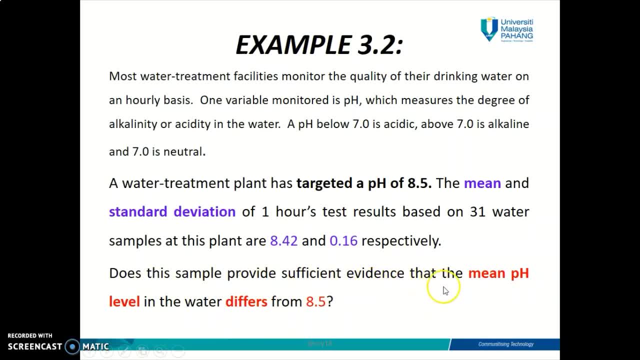 Does this sample provide sufficient evidence that the mean pH level in the water differs from 8.5?? So obviously this is our claim here: Mean pH level differs from 8.5.. So I think you all would already guess that this involves the expression of not equal. 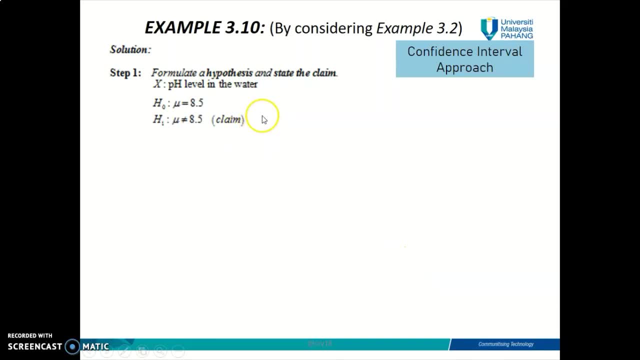 Alright, so let's go to the first step. We need to construct our hypothesis statement. So this is our claim here, Saying that the average pH level is different from 8.5, and then automatically you can construct your H now from here. Mu equals to 8.5.. 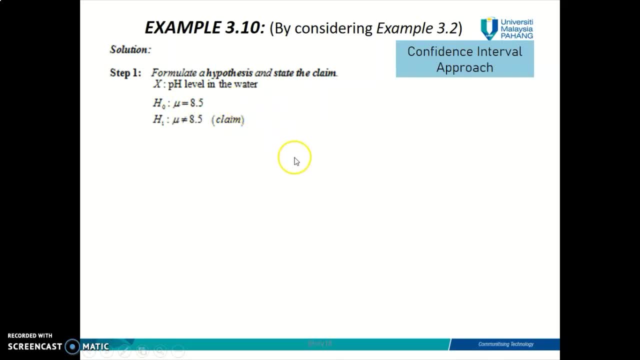 So I'm pretty sure that you're familiar with this first step. But the second step in confidence interval approach is to construct the confidence interval. Yes, So which confidence interval do you need to find in order to solve this hypothesis testing? So that highly depends on yourself. 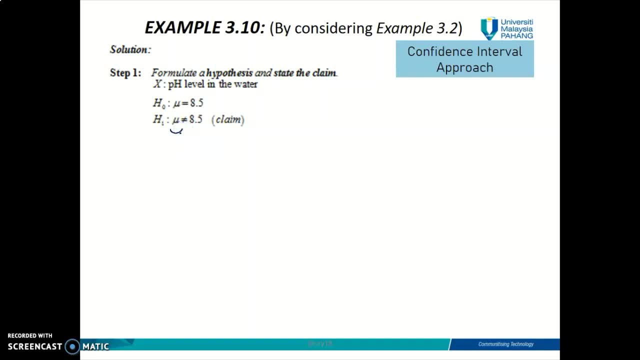 Let's say you are failing to solve step 1.. If your step number one involves one population mean, so the confidence interval you need to find here is the confidence interval for one population mean. Let's say your step number one involves 2 population proportion, So the confidence interval that you need to find in step 2 is the confidence interval for 2 population proportions. 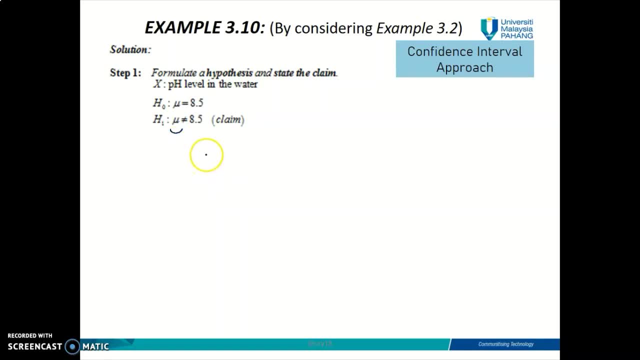 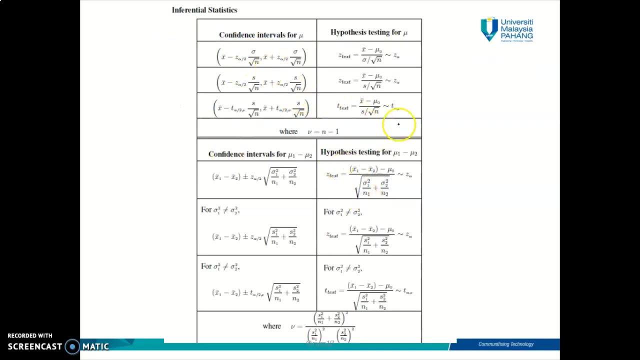 Okay, so let's try. let's go and find the confidence interval for our example 3.2. here I'm going to show you the formula table. okay, So in this formula book, right, these are all the formula for test statistics value. 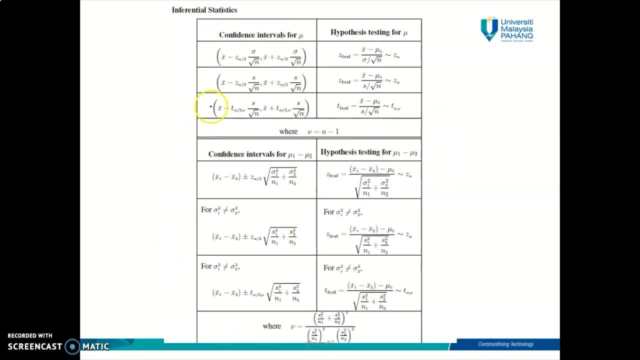 while the left-hand side here are all the formula that you can use to solve hypothesis testing using confidence interval approach. So please do not confuse between these two, okay? So let's continue to solve our example 3.2.. It involves one population mean. 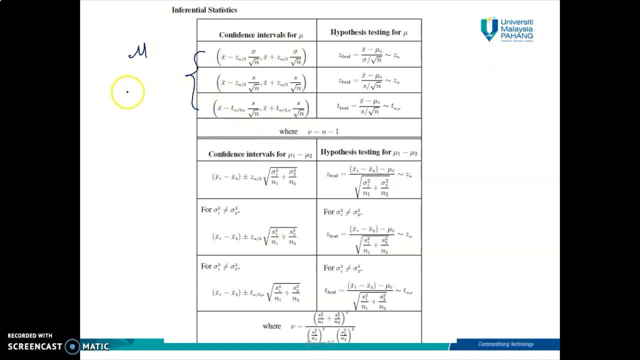 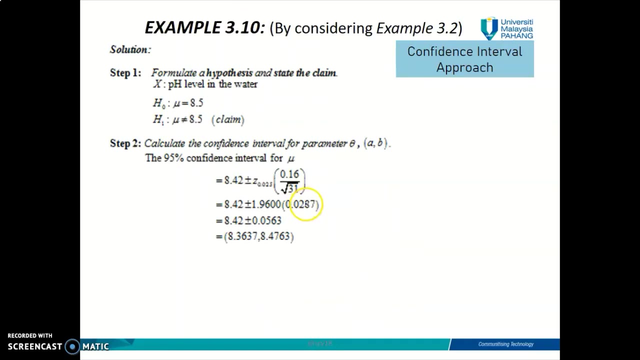 So I'm going to choose one of these three formulas here. And our example: just now: it is the case of sigma squared: unknown and sample size more than 30.. So this is the right formula for me to use, okay, So I'm going to continue and find the confidence interval, and this is the answer that I get. 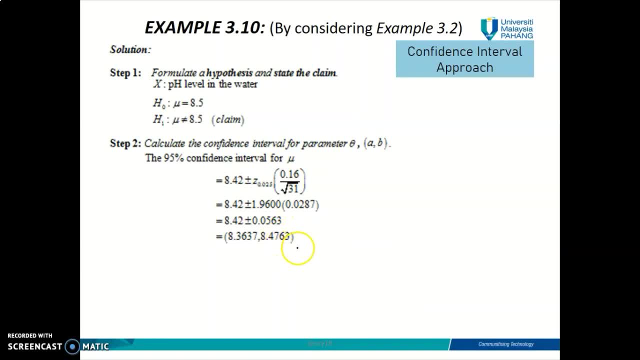 all right. So just substitute all the value accordingly and you will get the confidence interval here. So next We're going to make a decision based on our hypothesized parameter. okay, So let's recall what are the rules to make a decision in confidence interval approach. 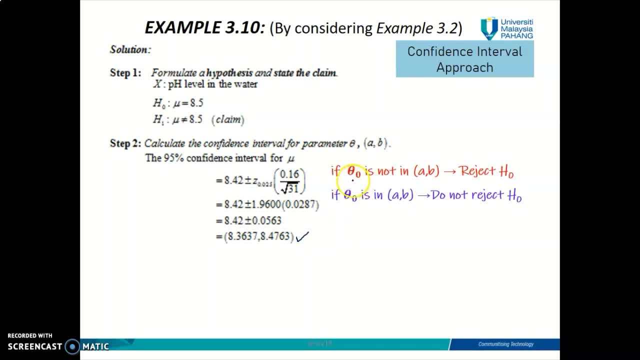 These two rules? okay. It highly depends on your hypothesized parameter. So what is your hypothesized parameter here? The hypothesized parameter in this case, here is our mu naught, okay, And I'm very sure that you know what is the value here. 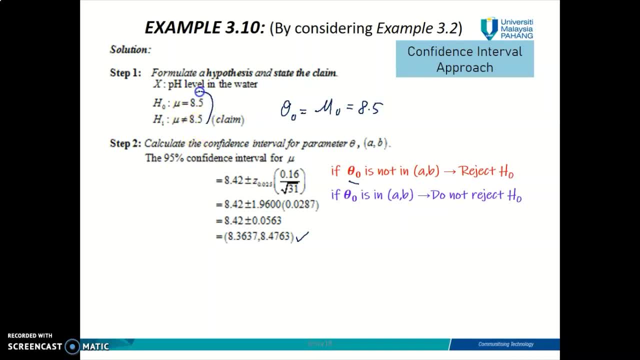 It is 8.5,. okay, It's the value That involves in your hypothesis statement. So now you need to look at this value here and you need to compare with. the confidence interval Is 8.5? within these two values? 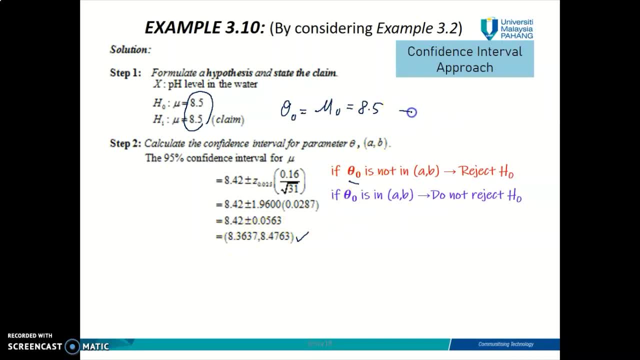 So how do you come to think of this? All right, So let's draw a number line. all right. So this is my a, my lower limit of the confidence interval, and this is my upper limit of the confidence interval. 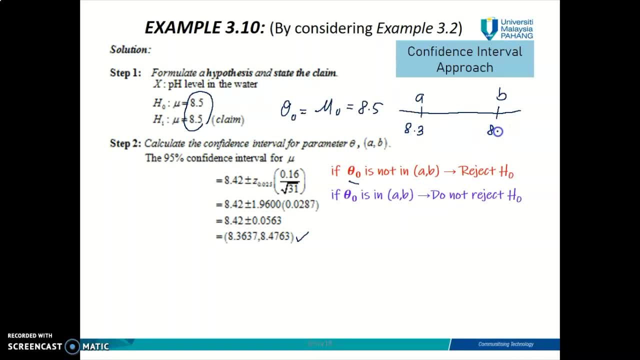 This would be somewhere around 8.3 and this is 8.5.. So the question now is: is 8.5 within a and b? If yes, so you will need to do not reject H now. If the mu naught is not within a and b, your decision would be to reject H now.